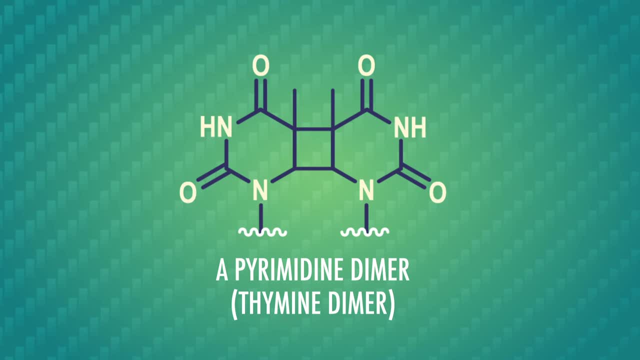 can react to form a ring structure. This is one type of paracyclic reaction. These now covalently bound bases called pyrimidine dimers can interfere with copying DNA and reading the encoded genetic messages, which can make things go pretty haywire, sometimes even causing cancer. 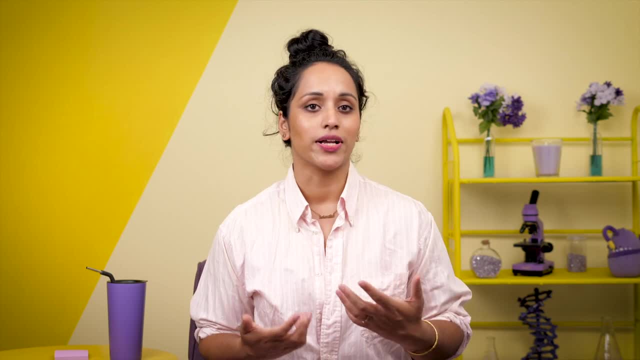 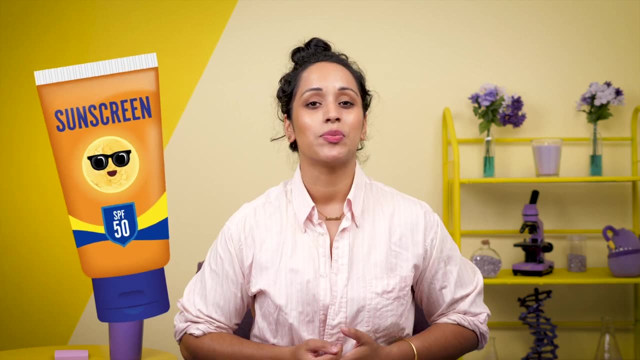 Because pyrimidine dimers are quite dangerous but also very common. our bodies have developed ways to remove and replace the damaged section of DNA, And we also use sunscreens to protect us from UV light. So in this episode we'll explore paracyclic reactions. 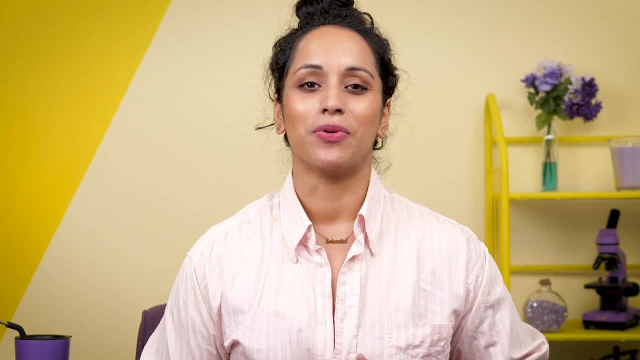 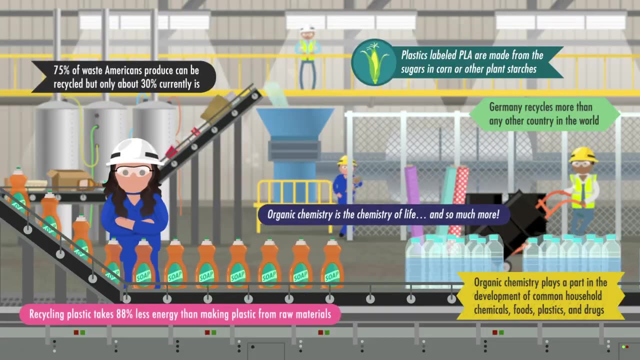 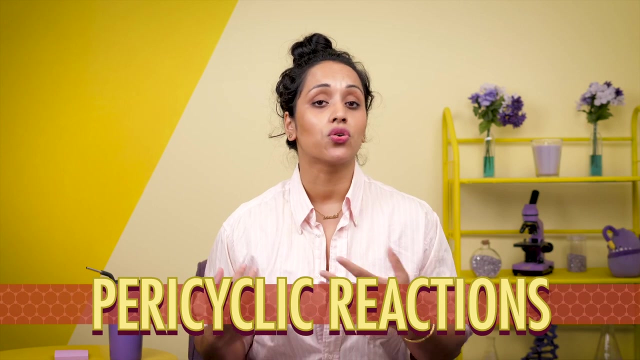 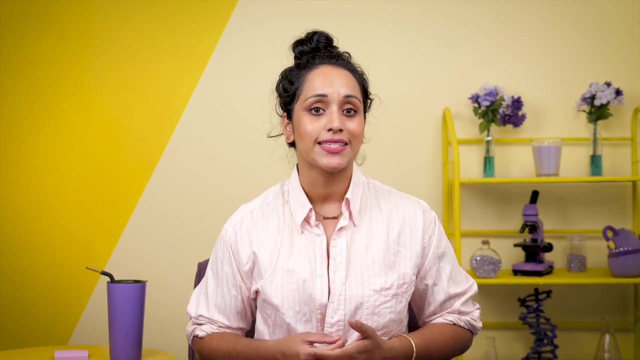 and how they relate to the sun's dangers and life-giving properties. There are quite a few paracyclic reactions across organic chemistry where overlap of molecular orbitals causes single and double bonds to break and form simultaneously in a concerted reaction. There's acyclic 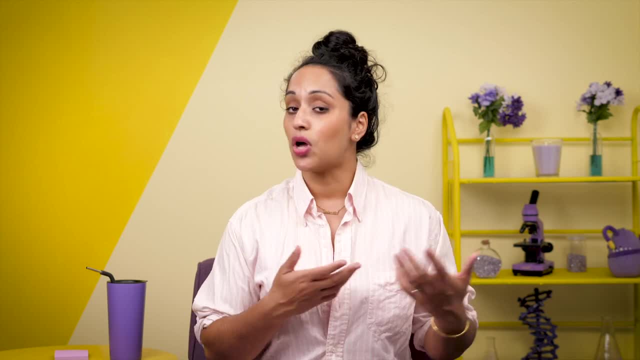 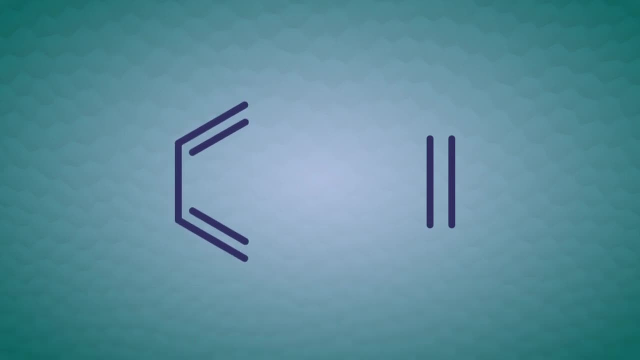 transition state but no distinct intermediates. It's all one step. A super important one is the Diels-Alder reaction, where a conjugated compound with two adjacent double bonds reacts with an alkene. This transformation makes two carbon-carbon bonds at the same time. 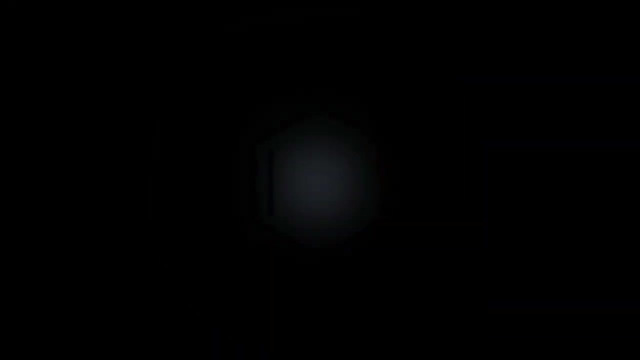 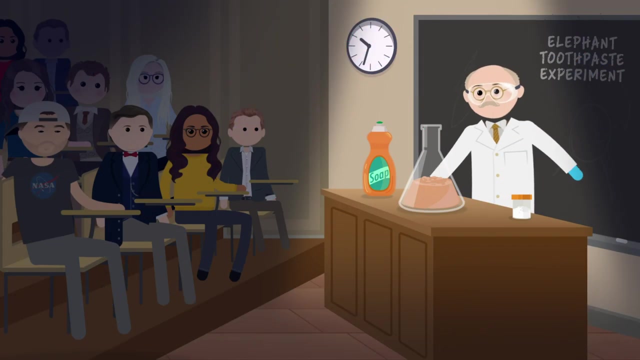 and shows incredible stereoselectivity and regioselectivity. This reaction bears the names of its discoverers and is a tale of a joint Nobel Prize awarded in 1950.. Otto Diels was a professor that cared deeply about research and teaching. 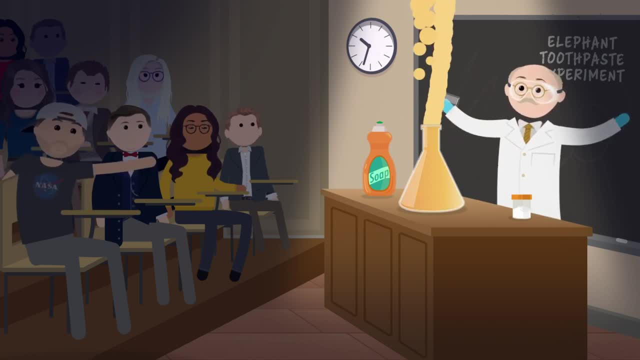 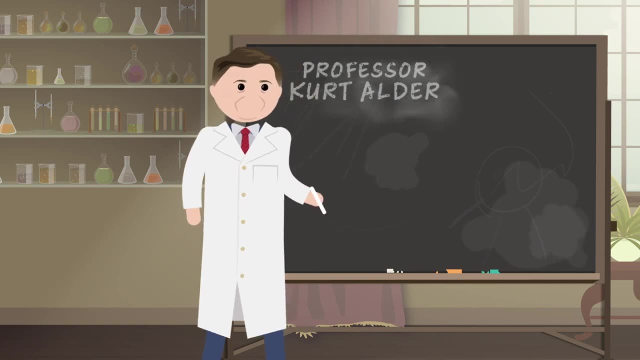 You'd find him demonstrating experiments at the front of lecture halls packed with hundreds of students at Kiel University in Germany. Kurt Alder was a student of Diels and became a professor himself after a stint in the rubber industry. He's also got a moon crater named in his honor. 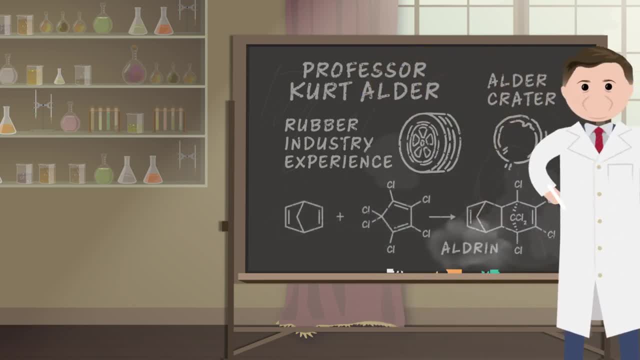 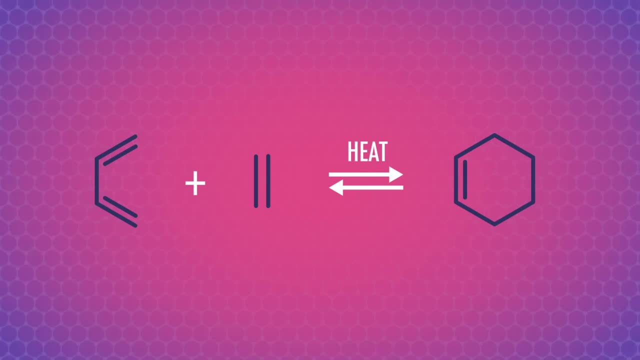 and the insecticide Aldrin, which is formed by a Diels-Alder reaction. In this reaction, our key players aren't just called a conjugated compound with two adjacent double bonds and an alkene. They have special names. The first reactant is a diene. 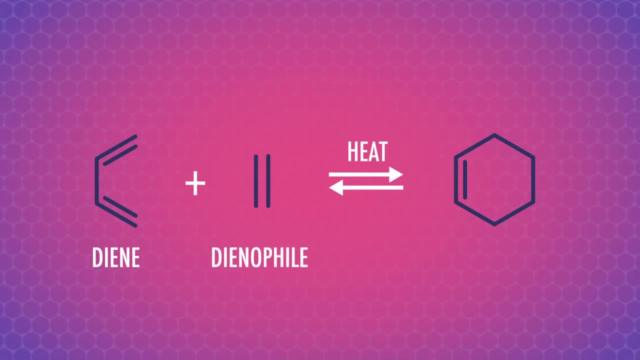 and the other is called the dienophile, the lover of the diene. Like we just mentioned, this mechanism is concerted and the bonds break and form at the same time. To show an arrow-pushing mechanism for the Diels-Alder reaction. 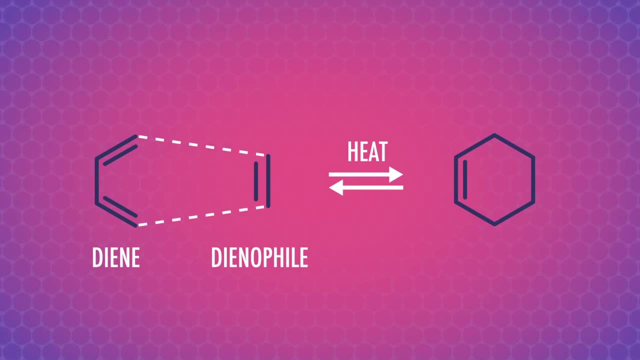 I like to draw dotted lines that connect each end of the conjugated system of our diene to each side of the pi bond in the dienophile. Now we can add three arrows to show the pi electrons forming new sigma bonds and a rearranged pi bond. 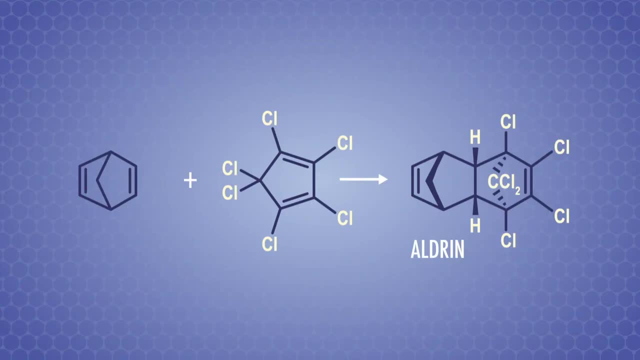 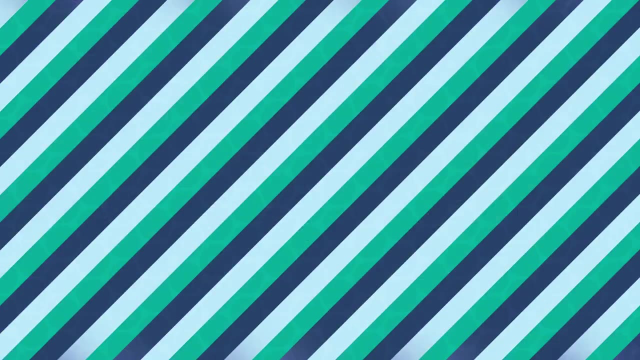 This helps me keep track of where to make the new bonds, even in more complex models. For example, if we want to make two new pi molecules like the insecticide aldrin, again we're sacrificing two pi bonds to make two new sigma bonds. 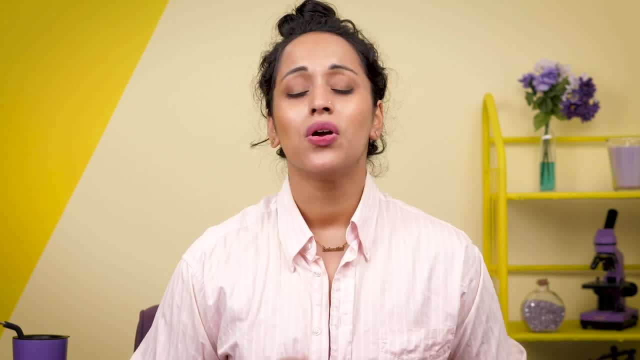 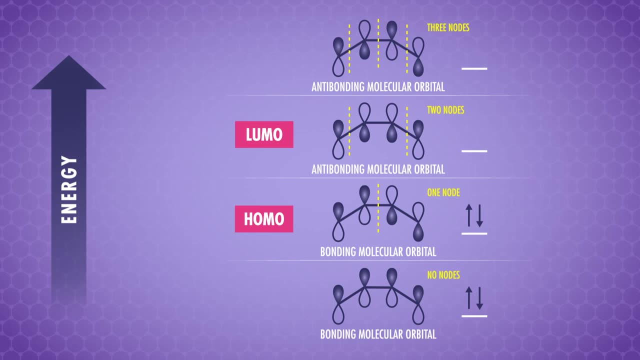 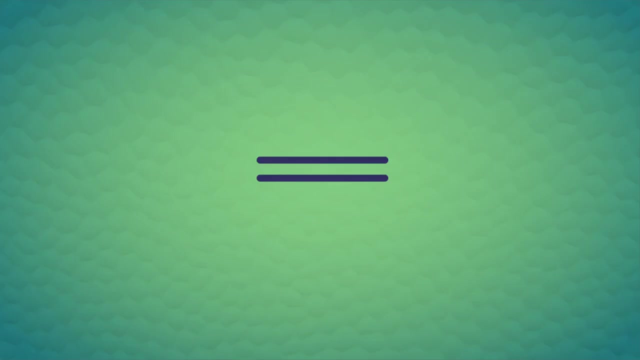 Now, even though we've been using arrow-pushing to help visualize how electrons move and form bonds, really molecular orbitals are what combine during a chemical reaction. Last episode we constructed the molecular orbitals of butadiene and these orbitals can be used to represent the pi system of any conjugated diene. 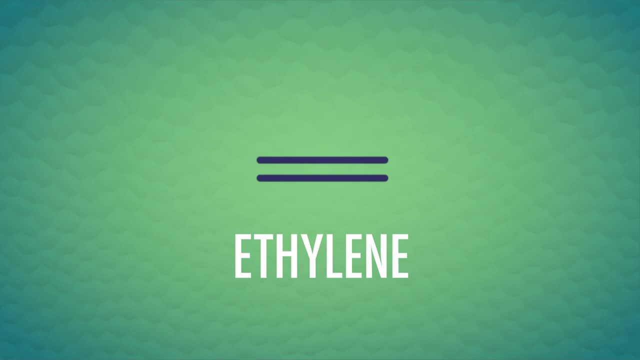 We can also construct the molecular orbitals of ethylene, which is the pi system of any dienophile. Ethylene has two electrons in the pi system. Those electrons pair up in the lower energy molecular orbital where we combine two p-orbitals in phase. 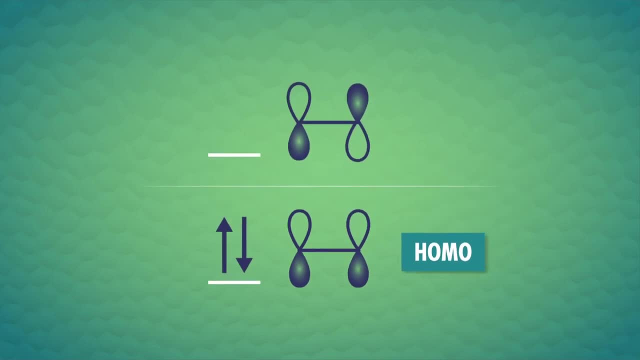 So this is the highest occupied molecular orbital, or HOMO. We can only construct one other molecular orbital by combining the two p-orbitals out of phase, And this is the lowest unoccupied molecular orbital, or LUMO. That's it. 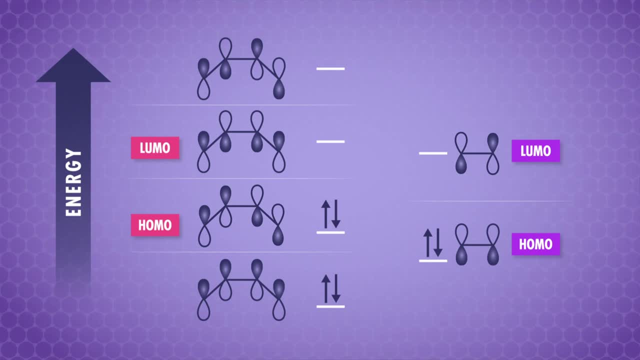 Now that we have the puzzle pieces, we can see how the molecular orbitals of a diene and dienophile can form a chemical reaction. In any chemical reaction, the HOMO of one reactant combines with the empty molecular orbital of the other reactant that is closest in energy. 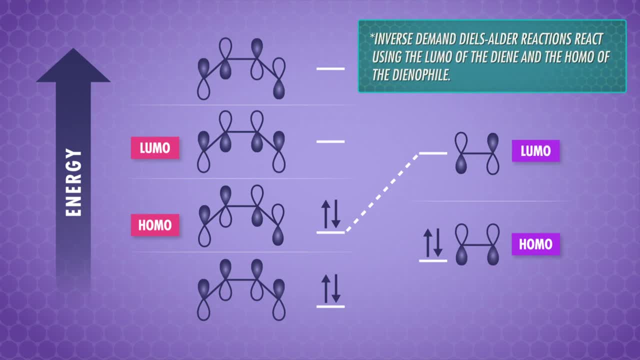 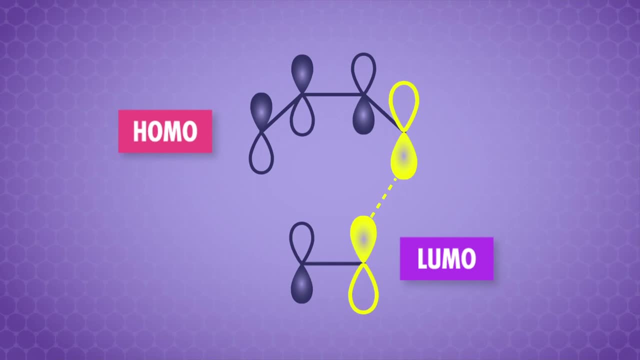 So usually the HOMO of the diene reacts with the LUMO of the dienophile. To be able to form new bonds, these orbitals need to be in phase. Look here: one shaded lobe of the HOMO lines up with the shaded lobe of the LUMO. 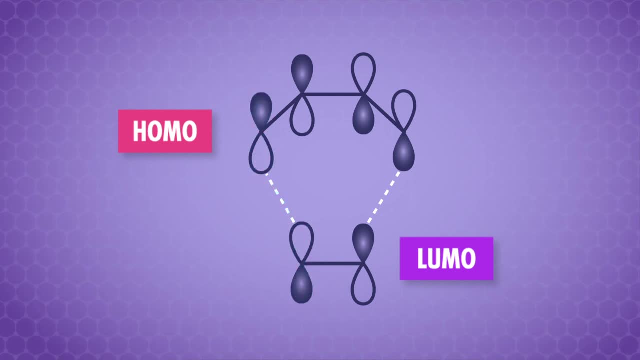 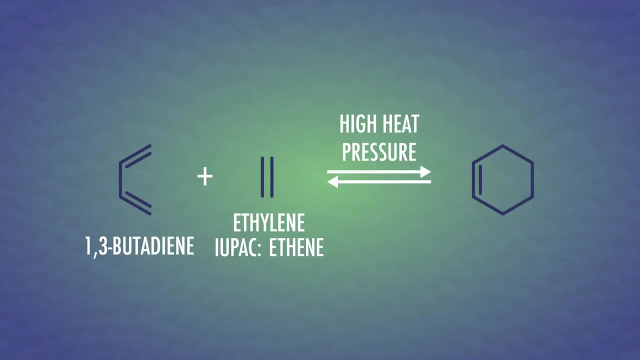 and on the other end the unshaded orbitals align, And when orbitals approach from the same phase, like in the Diels-Alder, they're superfacial. To be totally honest, the reaction of butadiene and ethylene to make cyclohexene is kinda terrible. 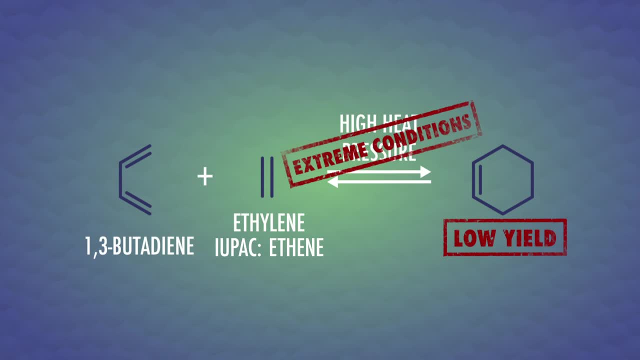 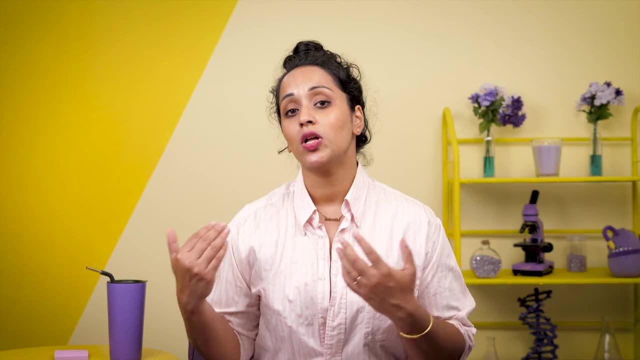 It happens under extreme conditions and in low yield. The HOMO of butadiene and the LUMO of ethylene are a bit too far away in energy, So to help most Diels-Alder reactions along, we'll put electron-donating groups on our diene and electron-withdrawing groups on our dienophile. 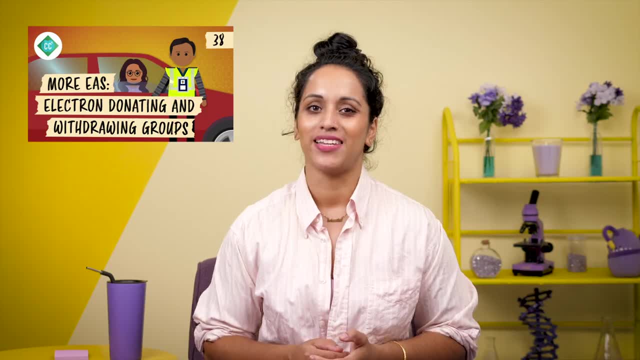 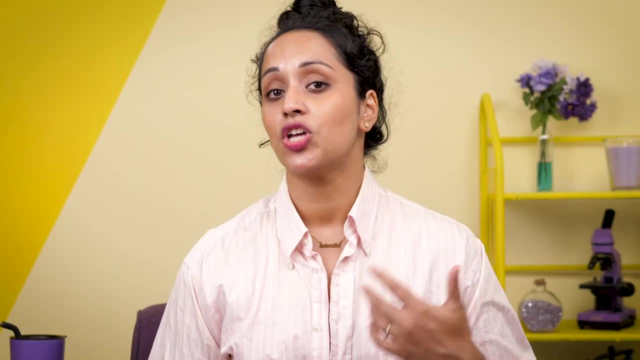 And for a refresher on how to recognize these groups, check out episode 38.. Electron-donating groups push electrons into the HOMO and it's energy, So putting these groups on the diene gets its HOMO closer to the energy of the dienophile's LUMO. 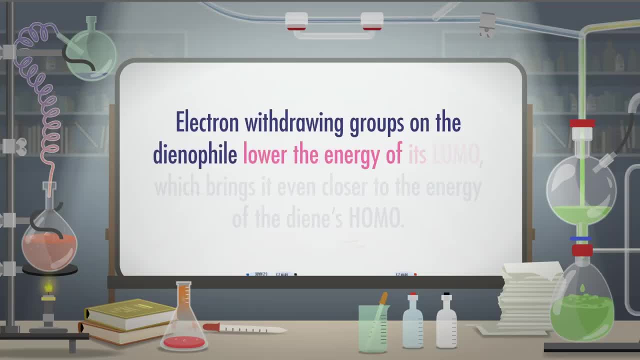 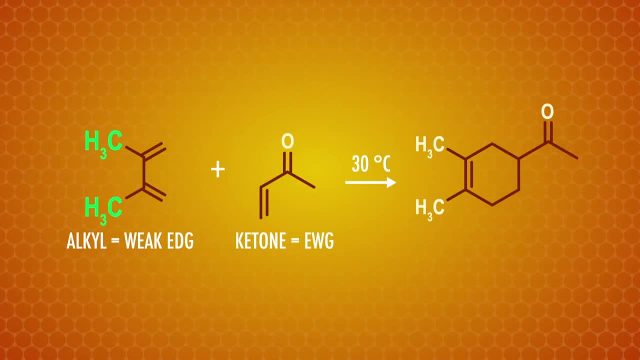 Electron-withdrawing groups on the dienophile lower the energy of its LUMO, which brings it even closer to the energy of the diene's HOMO. Let's look at a specific example, with weakly electron-donating methyl groups on our diene. 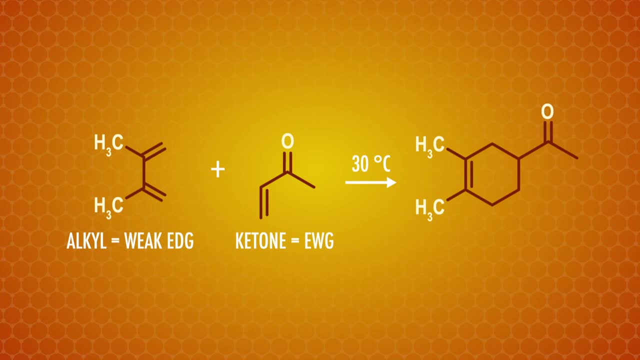 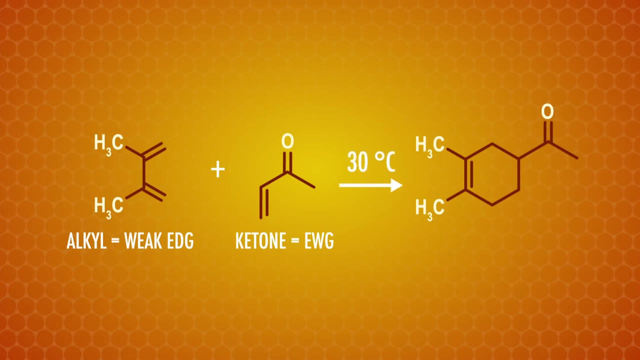 and electron-withdrawing ketone on our dienophile. With these groups, the HOMO of the diene is raised in energy, the LUMO of the dienophile is lowered and the reaction occurs with gentle warming, No extreme conditions here. 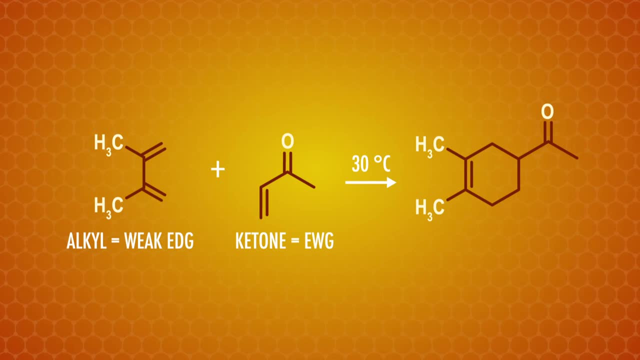 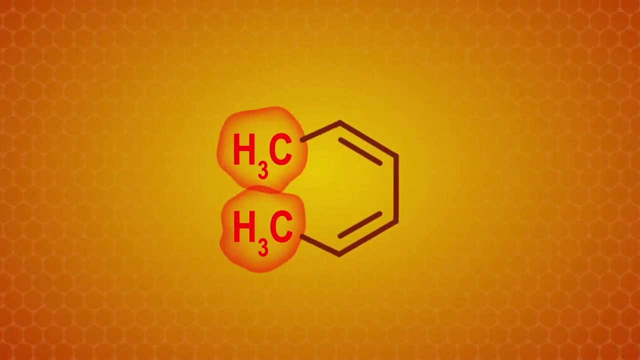 But we can't just stick electron-donating groups anywhere and expect chemistry magic. For example, this placement of methyl groups on this diene causes steric hindrance, so it can't adopt the reactive conformation and the Diels-Alder reaction won't happen. 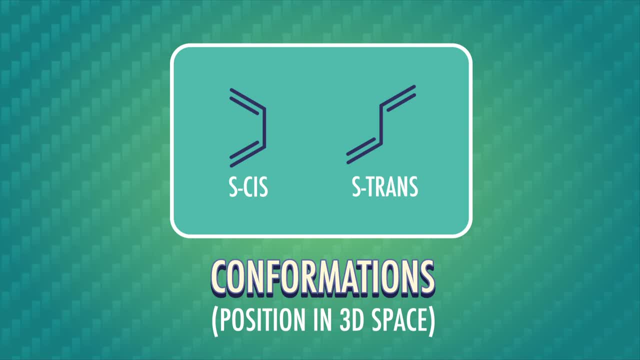 The reactive conformation with the double bonds ready to react is called S-cis And the unreactive conformation is called S-trans. The S at the beginning of these terms is really important, so we don't confuse them with cis and trans bonding groups. 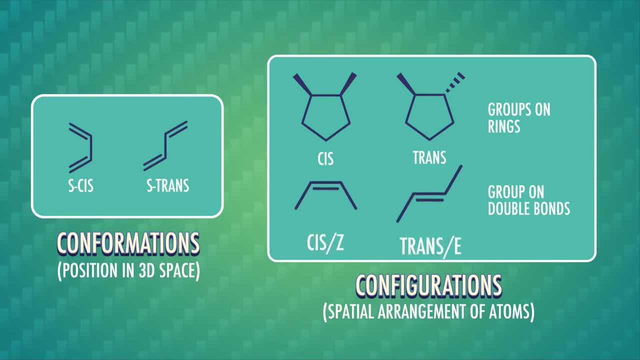 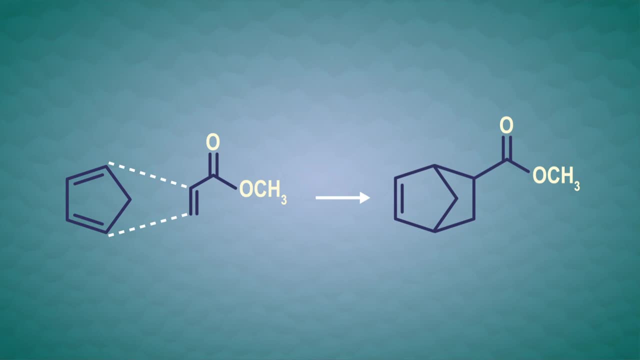 The S-trans is the reaction that's going to react to the double bonds, which, for double bonds, we've also been calling Z and E respectively. Compounds like cyclopentadiene that lock the double bonds in the S-cis configuration react well. 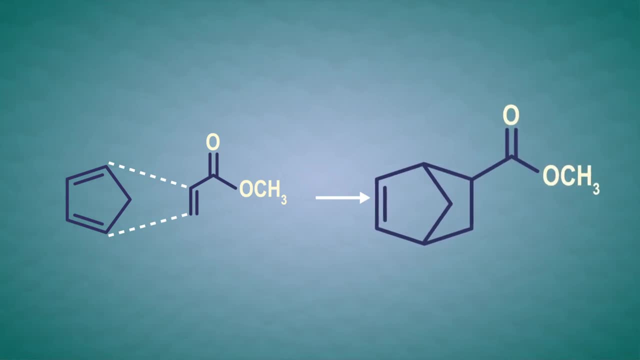 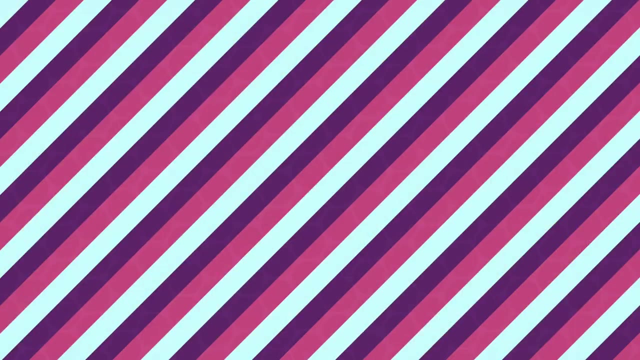 And because it's a ring already, the product of this example reaction is this cool double-ring bicyclic structure. Now that we know the basics of the Diels-Alder reaction, we can learn about its incredible stereoselectivity. First, we'll focus on alkene dienophiles. 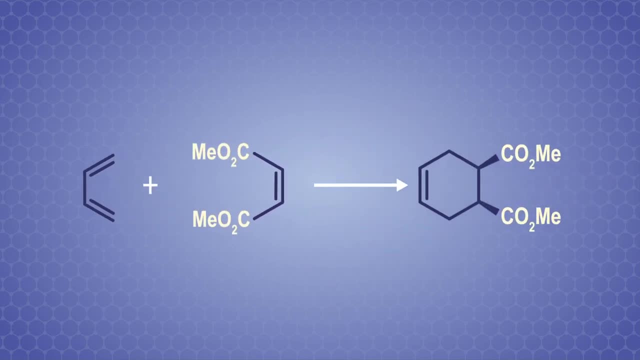 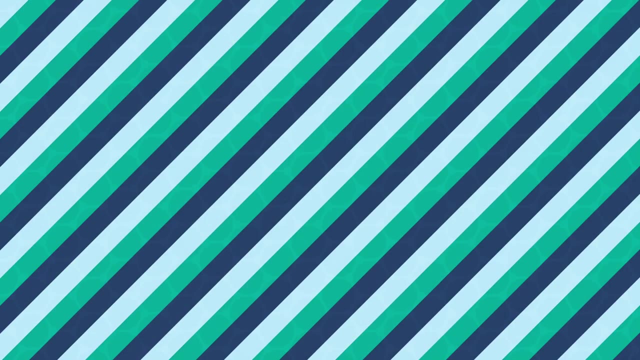 If the groups are on ze zame zide in a Z-alkene, they end up cis on the cyclohexene ring. And if the groups are E-cross in an E-alkene, they end up trans on the ring. Alkynes can be dienophiles too. In these Diels-Alder reactions the alkyne dienophile groups end up on a double bond, so they aren't cis or trans. Let's react an alkyne dienophile so we can look really carefully. 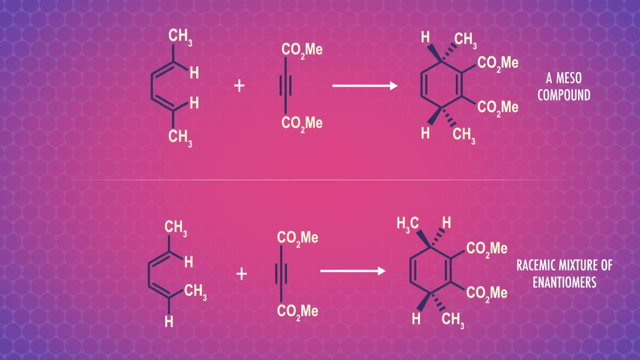 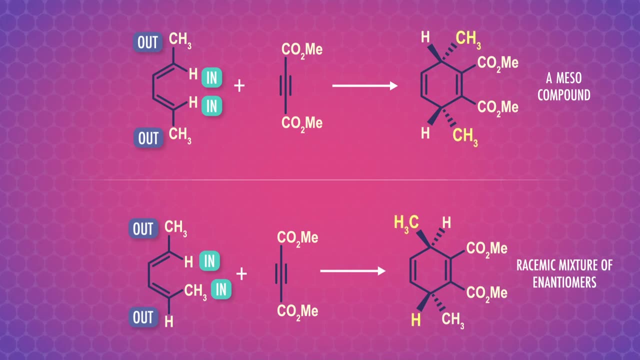 at where the groups on just our diene go With our diene in the S-cis conformation. we can label its groups out and in, depending where they're pointing The out. groups end up on the same side of the molecular plane. 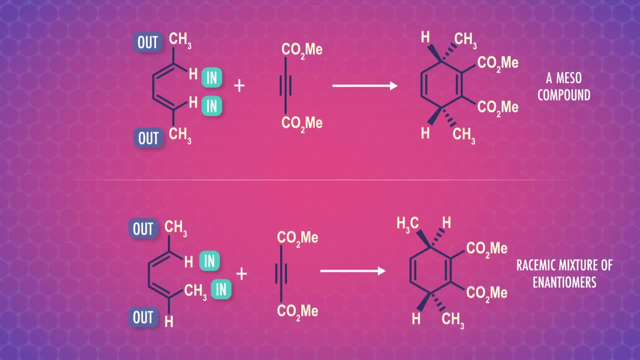 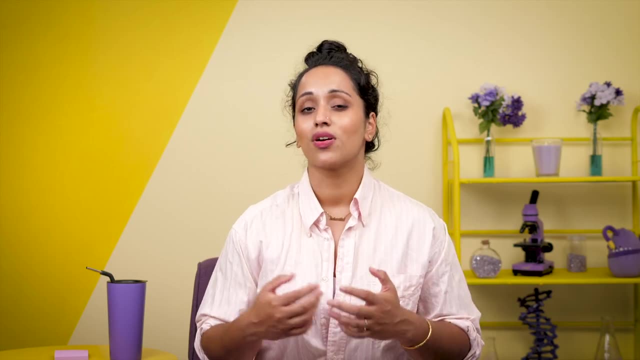 and the in groups on the same side. Remember, look carefully at the solid or dashed triangles that represent these bonds. But sometimes we're not only focusing on dienes or dienophiles to figure out stereoselectivity. We may see situations where both the diene and dienophile 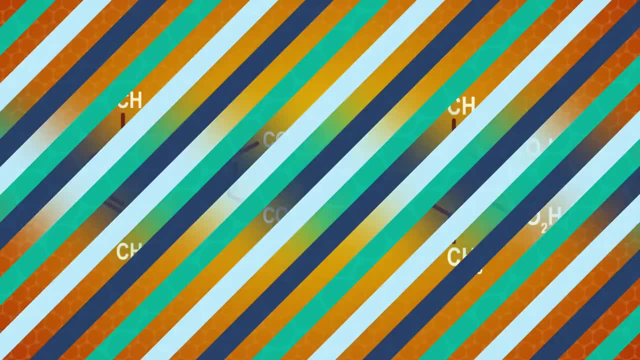 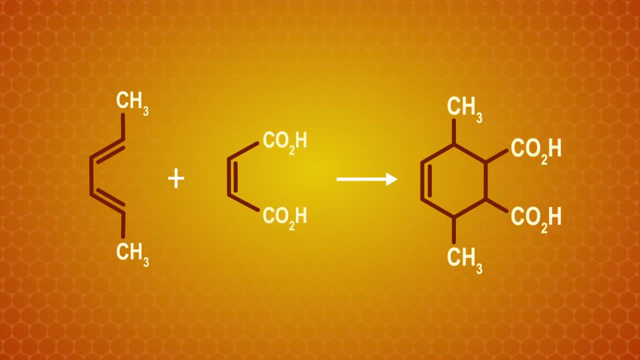 have groups that wind up on chiral carbons in the product, With the Z-alkene dienophile, for example. we know our carboxylic acids will end up on the same side And we know this diene has two out groups that will end up on the same side. 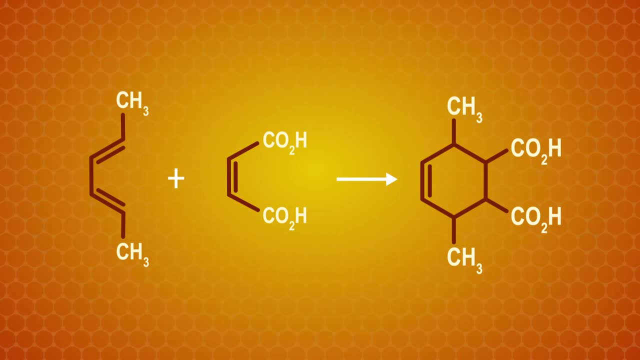 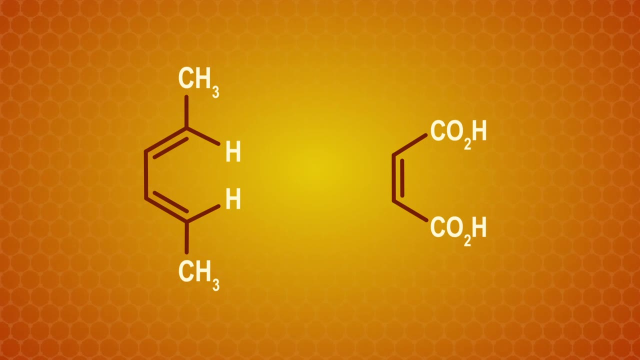 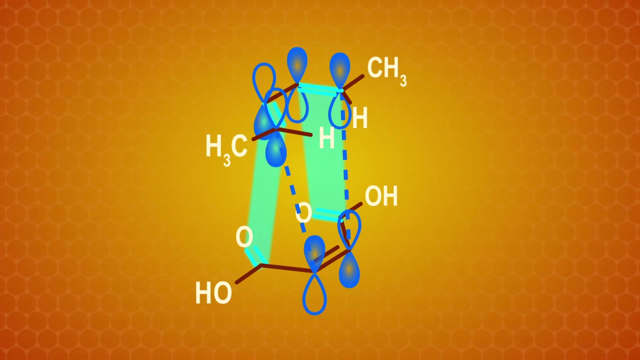 But what will the stereochemistry of the final molecule look like? The groups on the dienophile can have favorable interactions with the pi-molecular orbitals on the diene. So the dienophile approaches in this orientation, lining up the pi bonds in these carboxylic acid groups with the pi bonds of the diene. 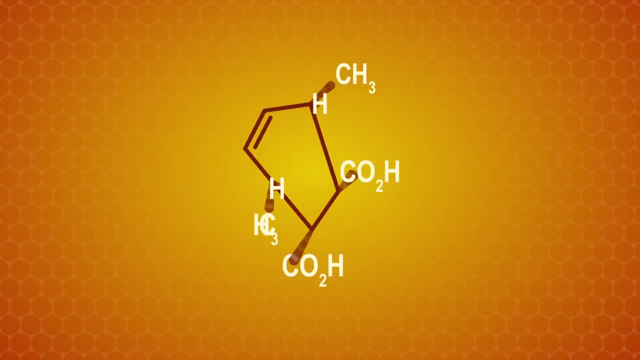 The bonds rearrange in our concerted Diels-Alder reaction And when we flatten out the molecule we can see it's this crowded product with all groups on the same side, And we know this diene has two out groups that will end up on the same side. 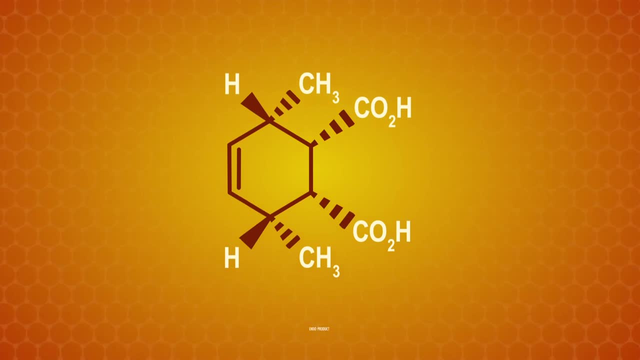 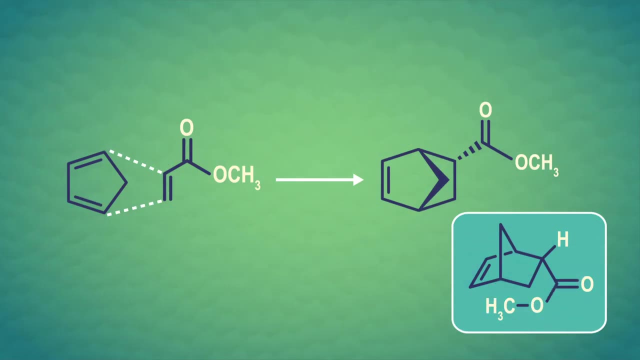 But what will the stereochemistry of the final molecule look like? This elbow-bumping molecule is called the endoproduct and the other potential diastereomer called the exoproduct is disfavored Bicyclic examples. let us see the endoproduct pretty well. 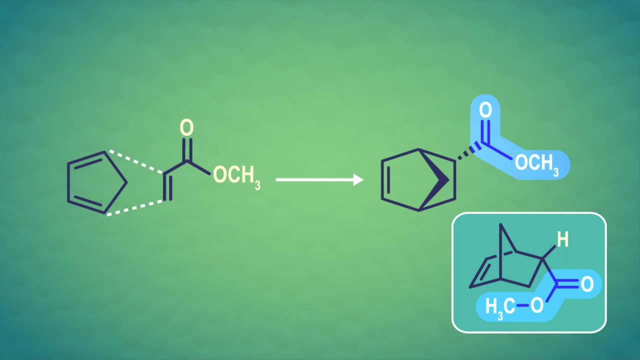 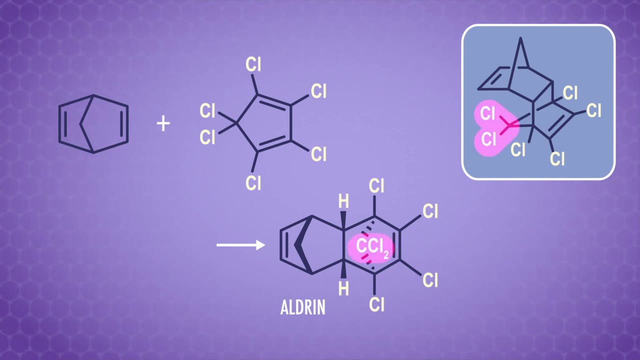 In this example, the ester points toward the more crowded side of the bicyclic ring. in 3D space And in our bicyclic insecticide Aldrin, we see the carbon-chlorine bridge faces the more crowded side too. 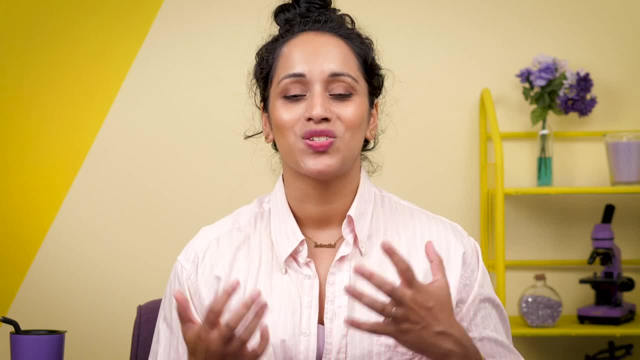 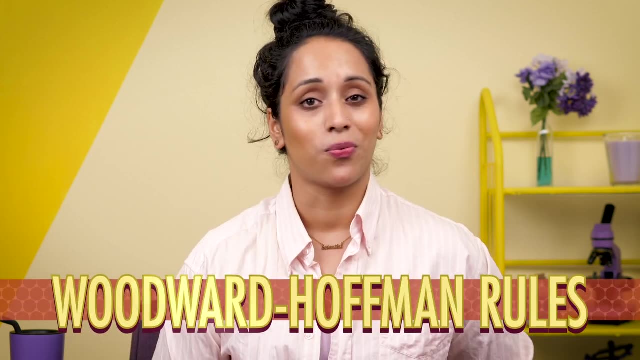 That's all we'll cover for stereochemistry, even though there's so much more to learn. If you're curious, the stereochemistry of all paracyclic reactions can be described with the Woodward-Hoffmann rules: A chain smoker with a propensity for blue neckties. 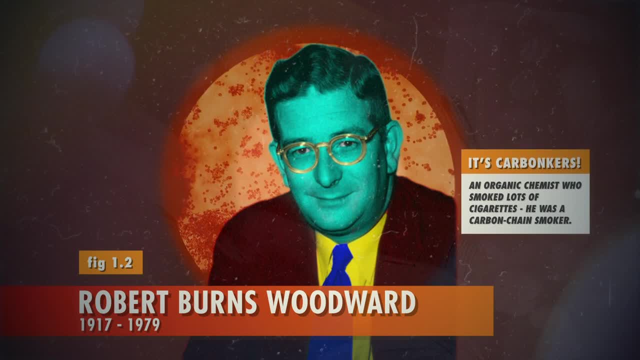 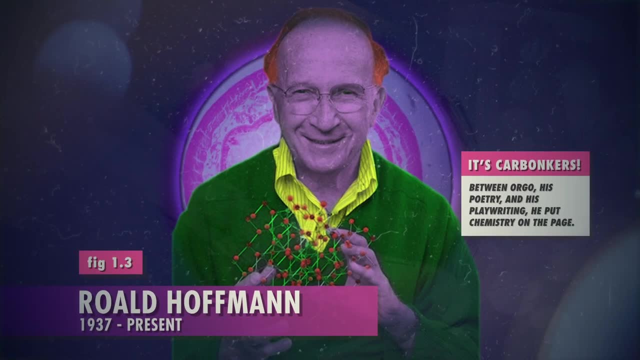 Robert Burns Woodward won the Nobel Prize in 1965 for the synthesis of complex natural products. He collaborated with Roald Hoffman, chemistry professor at Cornell University, to describe molecular orbital symmetry and predict the stereochemistry and regiochemistry of paracyclic reactions. 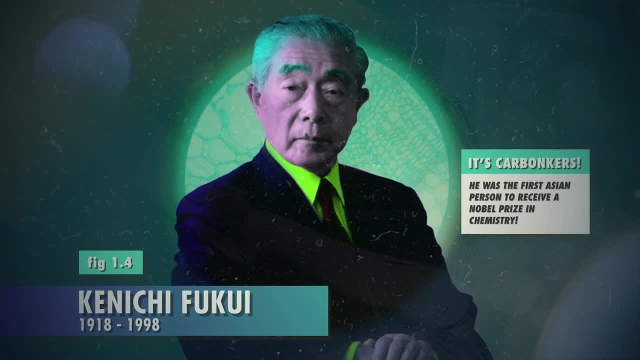 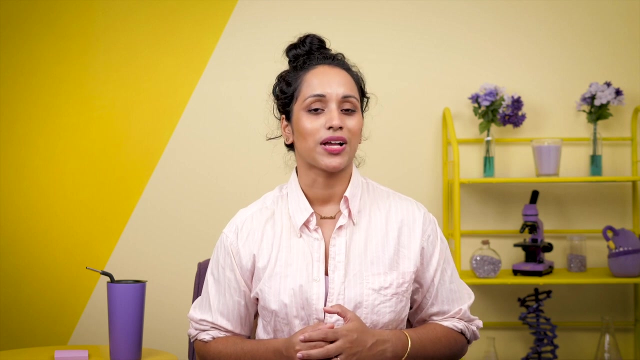 And in 1981, Hoffman shared the Nobel Prize with Kenichi Fukui, the first Asian person to win the award in chemistry. Their understanding of the influence of molecular orbitals on chemical reactions was a huge contribution to the field. Now we still have to talk about Diels-Alder reaction regiochemistry. 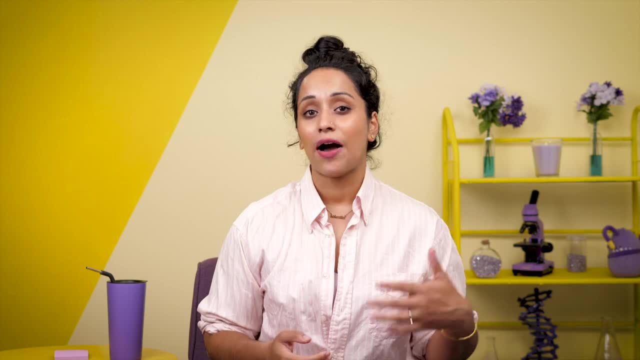 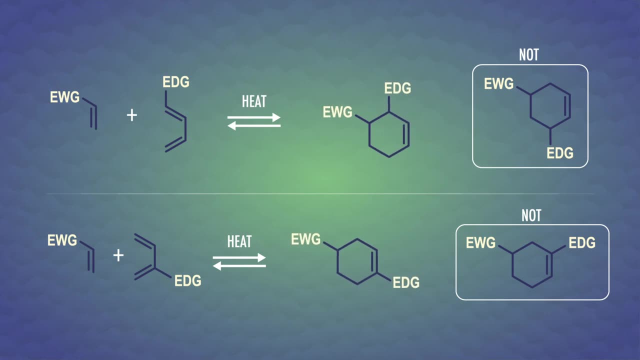 If we have one group on each reactant, we need to know how to predict where they end up relative to each other in the products. The groups in the products are actually kind of similar to the ortho and para positions on a benzene ring. 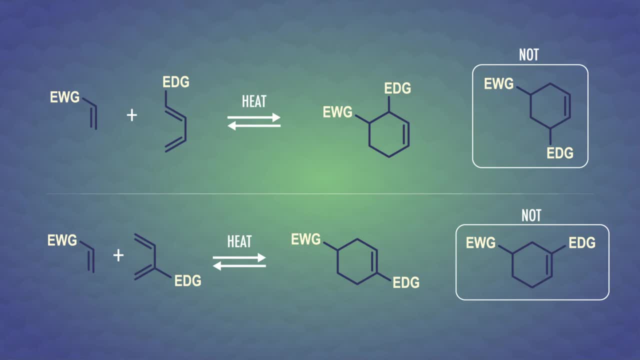 This is a cyclohexene, not a benzene, So this isn't official terminology, but it's a little trick that can help us remember where these groups end up. The position of these groups is actually dictated by the sizes of molecular orbitals. 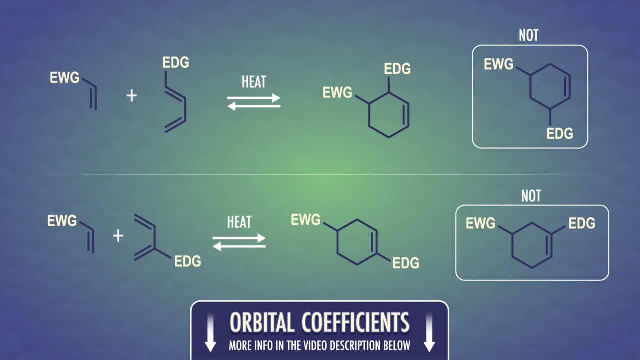 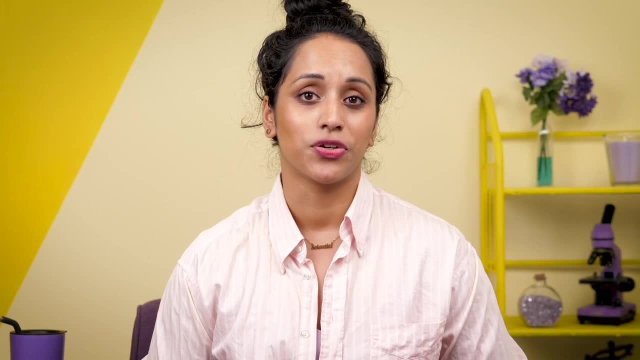 also called the orbital coefficients. We don't have time for that deep of a dive in this episode, but we've put extra references in the video description. We've been talking about the Diels-Alder reaction this whole time, but it's just one example of a cycloaddition. 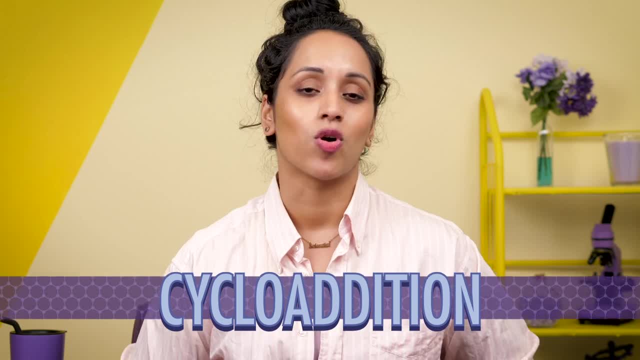 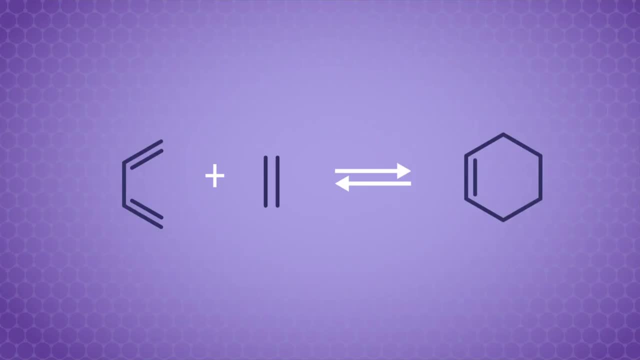 a type of ring-forming reaction where two new bonds form simultaneously. Cycloadditions are classifications and they're classified by counting the number of carbons in the pi system in each reactant. So the Diels-Alder is a 4 plus 2 cycloaddition. 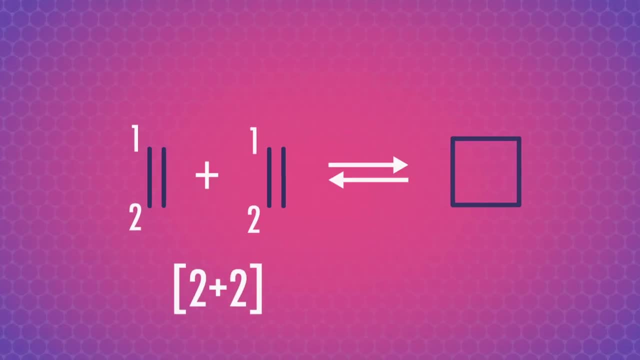 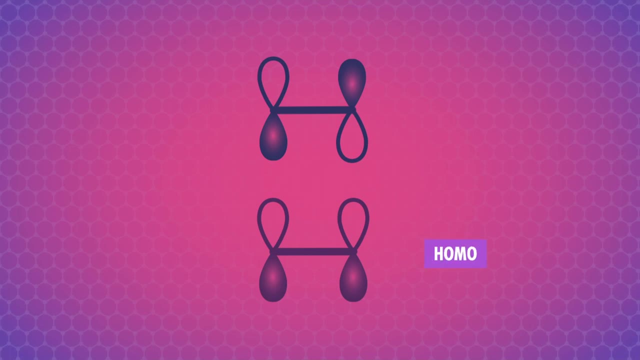 The pyrimidine dimers we saw at the beginning of the episode are a 2 plus 2 cycloaddition and we can draw arrows for the mechanism like this. But looking at the molecular orbitals… wait a second. The HOMO of one ethylene molecule doesn't line up with the LUMO of the other. 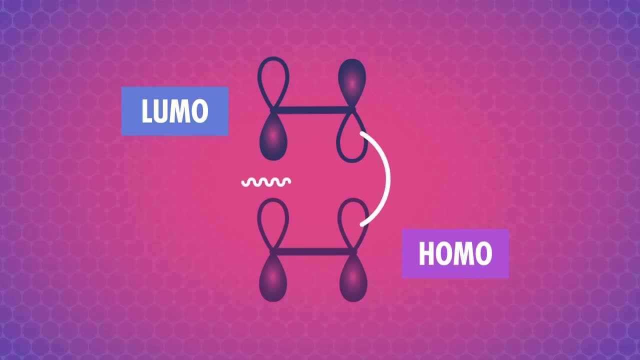 This isn't superfacial like the Diels-Alder reaction, because one of the two pairs of orbitals doesn't line up. In fact, the antarafacial or opposite-face approach that would be required because of the not-in-phase-ness won't. let us form new bonds. 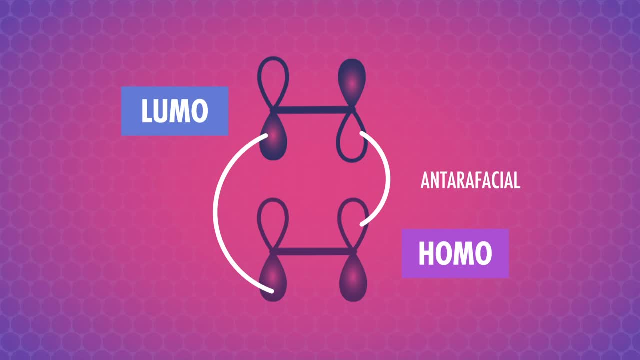 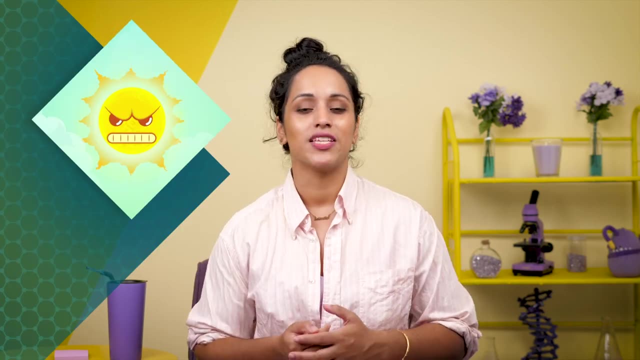 The rigid double bonds don't let our ethylene molecule reach the opposite face. So what do we do? Don't forget we have another key ingredient – sunlight. Just like with UV-vis spectroscopy, the UV light excites an electron in one reactant to the next energy level. 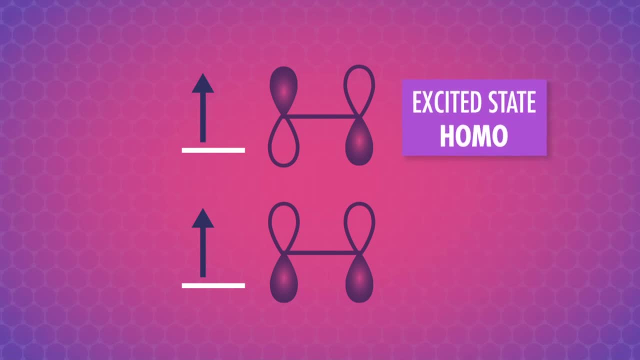 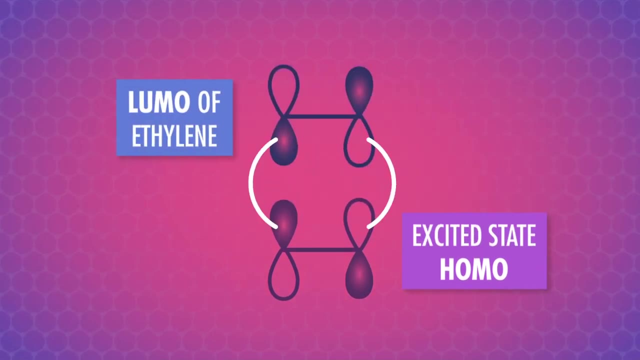 so it has a new HOMO. You can review this in episode 41.. Let's start by lining up our orbitals for the 2 plus 2 cycloaddition. again, They're in phase and superfacial now, So with UV light, 2 plus 2 cycloaddition can occur.